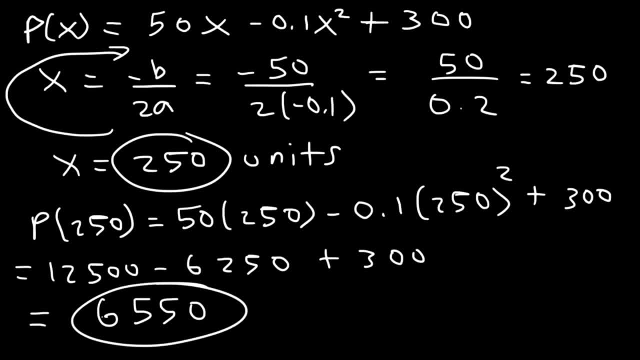 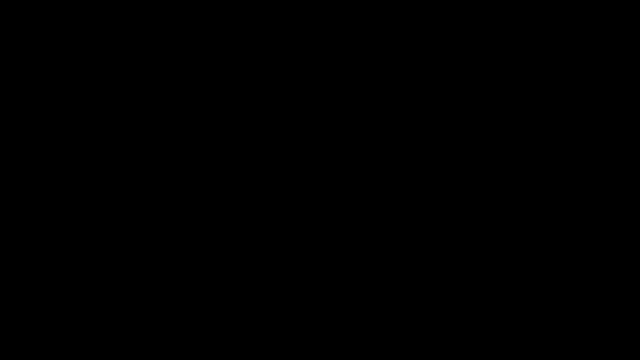 is 6,550.. And that's it Now. the next type of word problem that you might see associated with this chapter is basically projectile motion, which is a physics topic, But you can use algebra to solve Certain aspects of it. So let's say that the height of the ball can be modeled by the function. 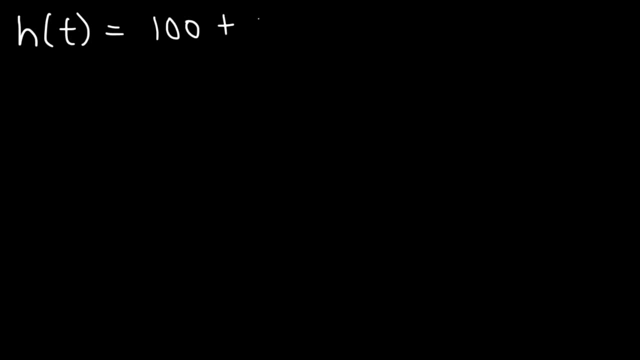 H of T, which is 100 plus 30 T minus 4.9 T squared. Let's say T is in seconds and the height is in meters. 100 represents the initial height, So chances are the ball is kicked off from a cliff. 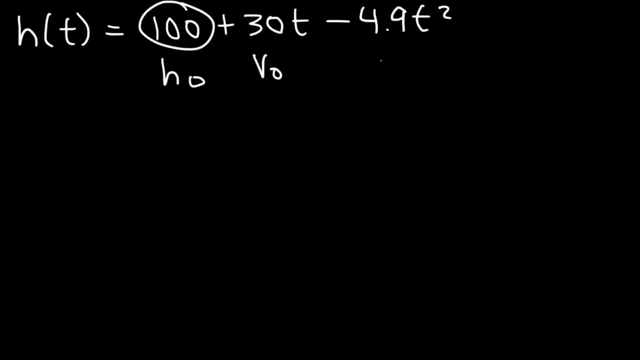 30 represents the initial height, 40 represents the initial velocity And 4.9 is really the combination of one half and the acceleration due to gravity, which is 9.8 meters per second. So just some background info on the equation, if you wanted to know. 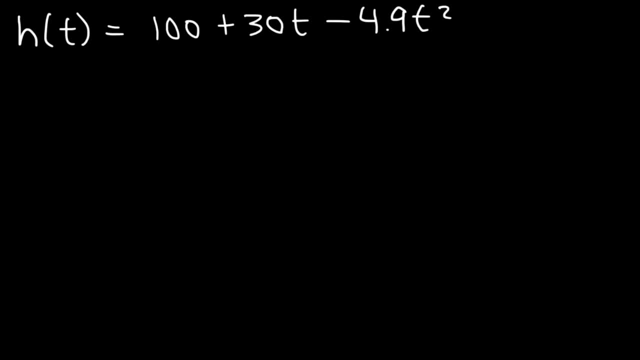 But we really don't need to know that. Most problems of this type will typically ask you: how long will it take for the ball to reach the maximum height, and what is the maximum height? The equation that you need to know is the following: 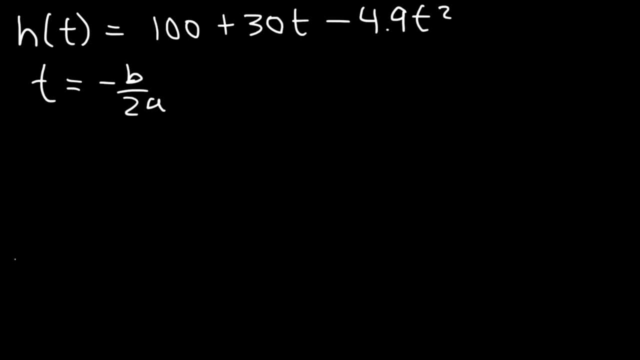 Negative B over 2A. Here is a picture, if you want it. Let's say: that's the cliff And here's the ball. It goes up and then it goes down. So we want to find the time it takes to reach the maximum height. 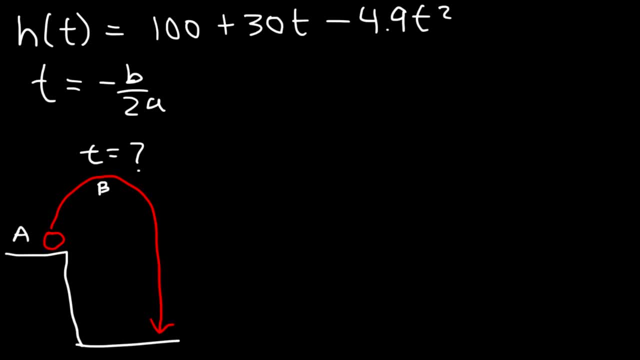 How long does it take to get from point A to point B? And we want to find the maximum height, which is the distance between point B and ground level, which we'll call point C. We also want to find the distance between point B and ground level, which we'll call 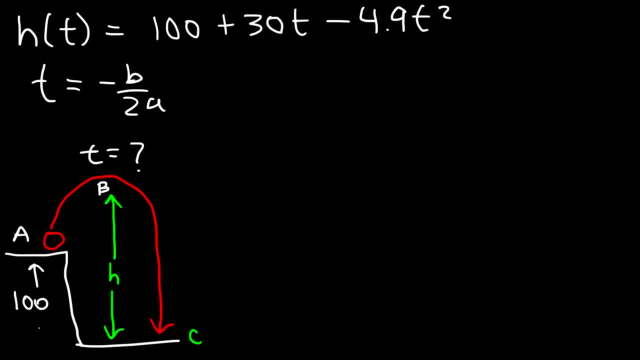 point C, which is basically the height of the cliff or the height of the building, that's 100.. So now let's use this equation. So B is the number in front of T, that's 30.. A is the number in front of T squared, which is negative: 4.9..